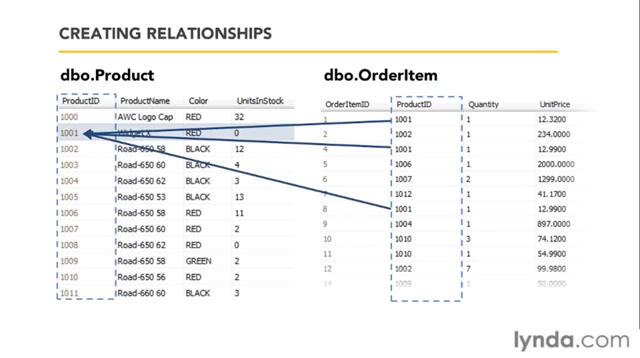 for example, the product ID: one, zero, zero, one, three times in order items, or four times, or a dozen, all referencing the same product. We could have 1010, pointing to our 1010 product. We could have 1002.. This is the relationship that we're talking about. 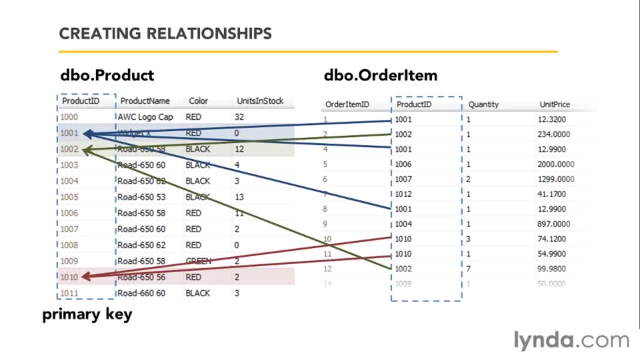 between our tables. In the product table, product ID is referred to as the primary key. It is unique. In the order item table, product ID is referred to as a foreign key. It's a key to some other table, allowing us to join our information together. The benefit of having this relationship. 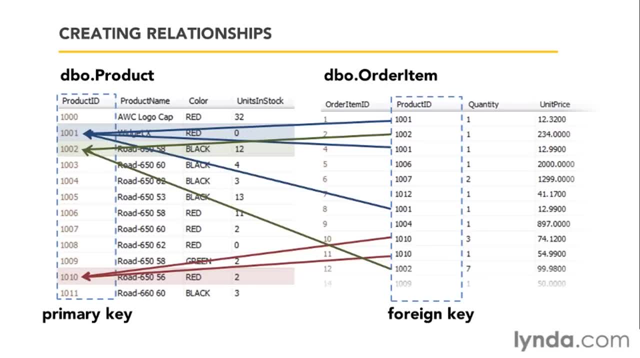 described is we can go either way. We can go from the order item and go and get product details, or we can go from the product and find how many order items have been created for that product, And when you have a relationship like this, it's what's defined as a one-to-many relationship. 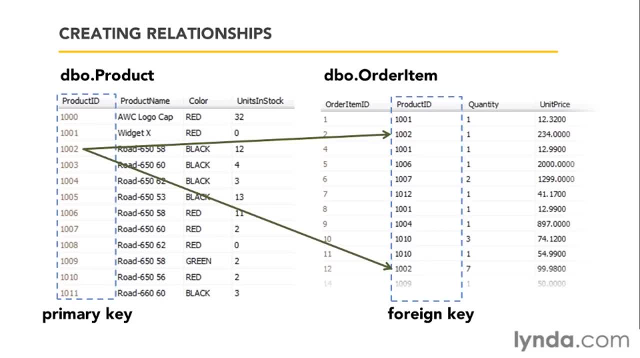 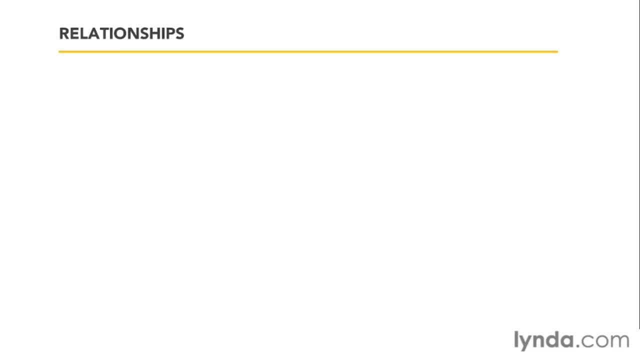 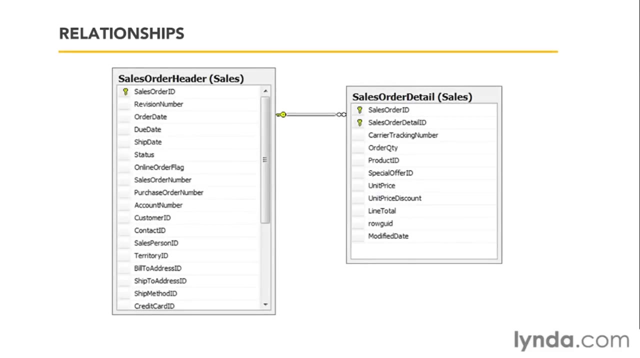 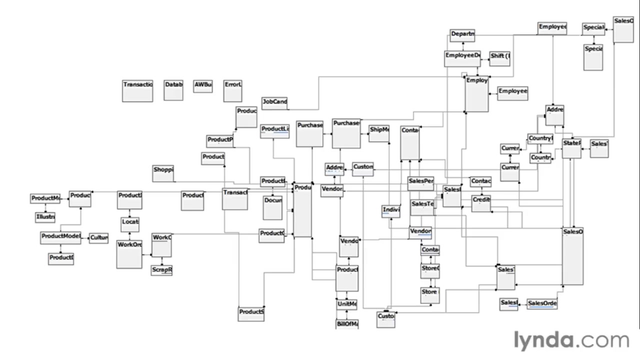 or potentially hundreds of relationships when you design your databases. If you're using SQL Server Management Studio to show a database diagram, you'll actually see that relationship defined between the tables And as you create more and more complex databases, you'll find that you're going to have relationships between most of them. What I'm looking at here is just a zoomed 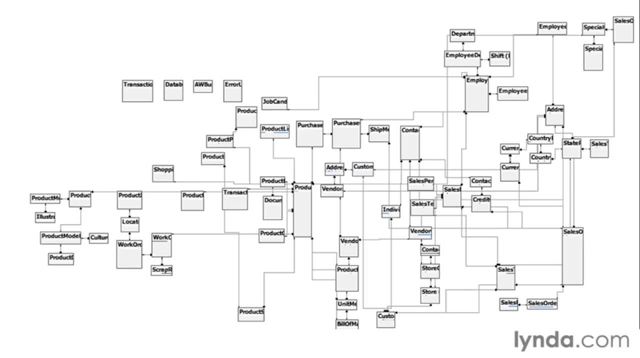 out diagram of the AdventureWorks database, And that's not even a particularly large database. So it's very, very common to have relationships between your tables, And the reason why I'm saying that is because there really are two main kinds of relationship that we care about. 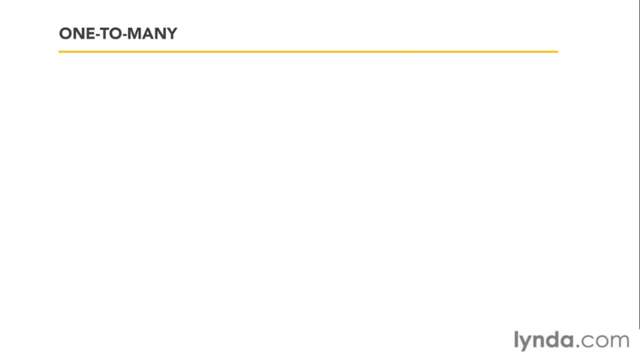 The first one, the most common, what we just explored, the idea of a one-to-many relationship. So one customer, many orders. One category has many products in it. One department has many employees. Now, bear in mind, when you describe a one-to-many relationship, you don't actually. 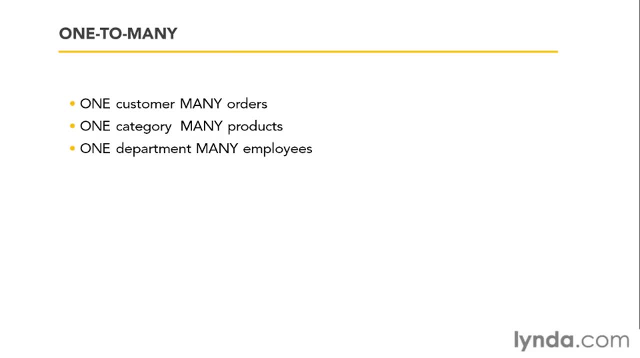 have to have many, meaning one customer might only place one order, might even place zero orders, But one customer can have many orders, One category can have many products, One department can have many employees, But the important point is here that, at least according to your own business, 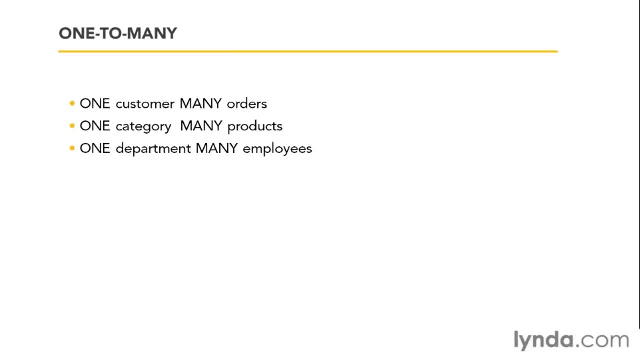 rules. the opposite of these statements is not true. That in your business an order has one customer, You don't say: yeah, an order can have many customers, It can't. An employee has one department, A product has one category. So you can view this either from the top down or the bottom. 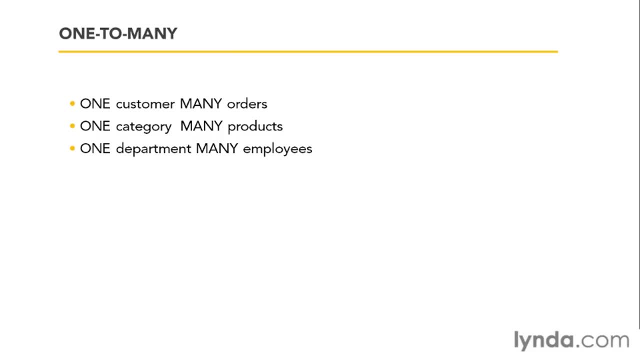 up whatever makes sense Now, as this is the most common thing that you're going to see. when you're looking at a diagram in SQL Server Management Studio, you'll see the relationship defined like this: with this icon: The key represents the one and the infinity sign represents the many. So when you're looking at this, 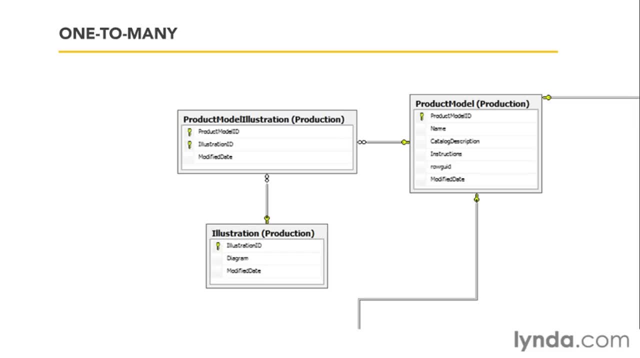 diagram. it doesn't matter whether the tables are shown on top or underneath. What's important is where the key is. The next kind of relationship that we can have is called a many-to-many relationship. It's not as common as one-to-many, but it's still. 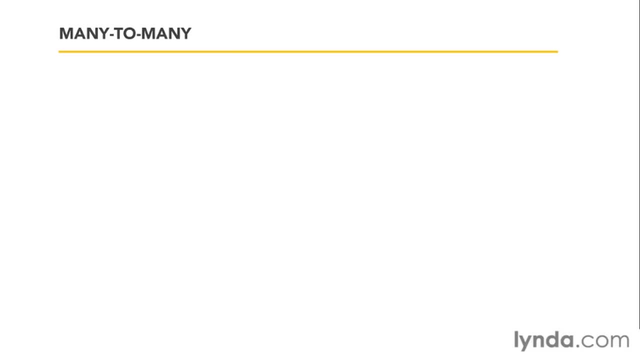 quite common. Now you often have to think about this one, because these business situations can often feel like one-to-many at first. Let's say we have an author table with a list of a few authors inside it and their names and some kind of key and identity for them, And we also have a title. 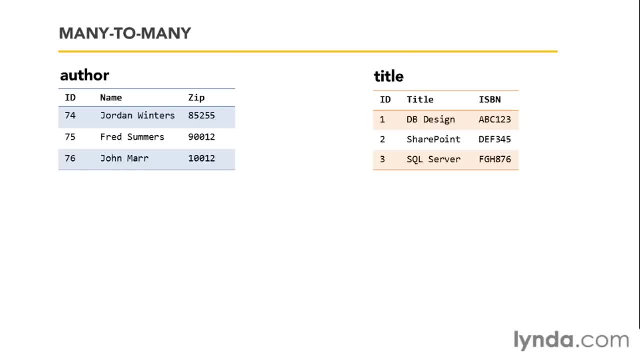 table with a list of book titles. Well, at first glance, what we might say is: okay, this is a one-to-many relationship. We could take the author number 74,, Jordan Winters, and we could take the author number 74, Jordan Winters and say that we want to represent that author has written both. 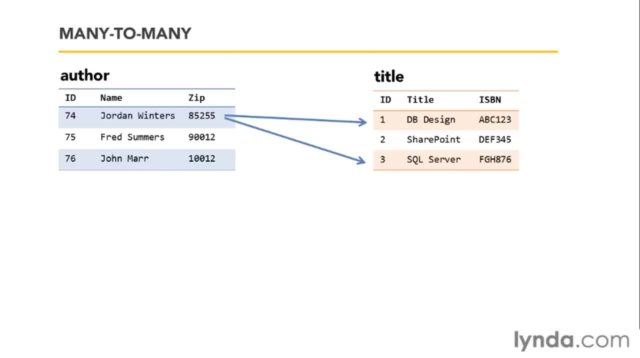 book 1, DB Design and book 3, SQL Server. And we can say that Fred Summers- author number 75, wrote book 2 on SharePoint. And if this was a classic one-to-many relationship- one author, one or more. 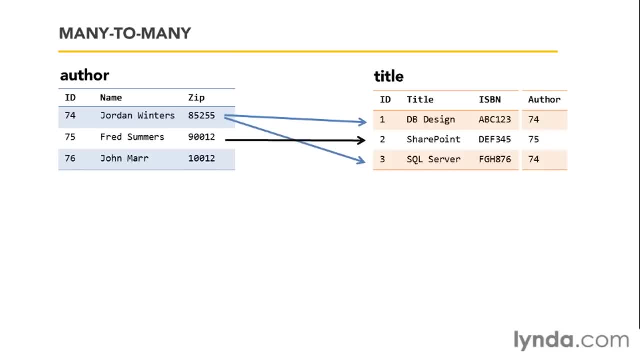 titles. we could add a new column to the title table. This would be an author ID column. It would be a foreign key to the author table. But here's the issue: What happens if in a day we have a, or a week or a month? we say, well, actually the SQL Server book was written by two authors. 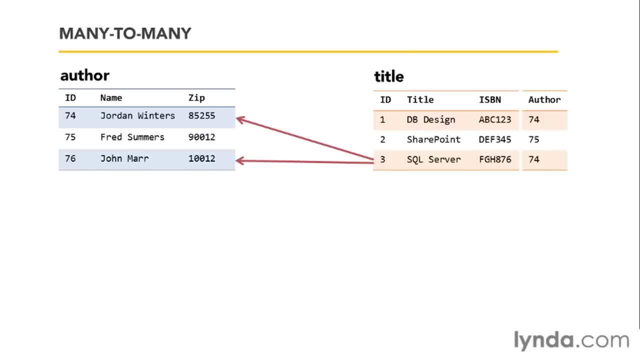 Well, the way that we have it right now we have that author column can only store one. It's storing a foreign key to author ID 74. And this is what we mean by a many-to-many relationship. One author can have many titles, One title can have many authors. Now, the way some people try, 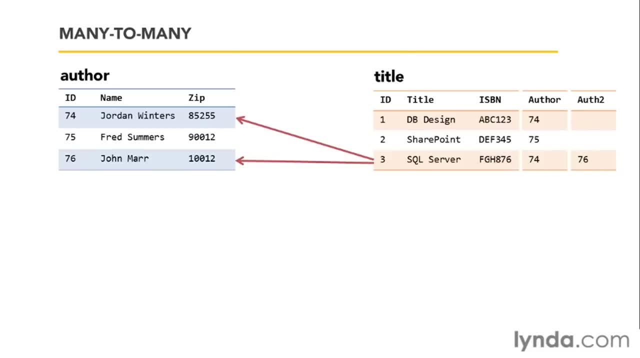 and model. this is: they'll add a new column to the title table. They'll put in author 72. And they'll have that be 76 and point it to John Marr. However, adding new columns to your tables, and particularly these kind what are called repeating groups or repeating columns, 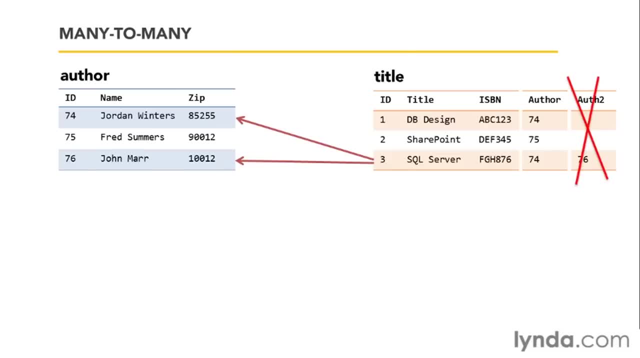 is a really, really bad idea And it's a definite no-no in database design. So we'll get rid of that idea. Well, some other people think: well, I'm going to cheat a little bit And I'll just do. 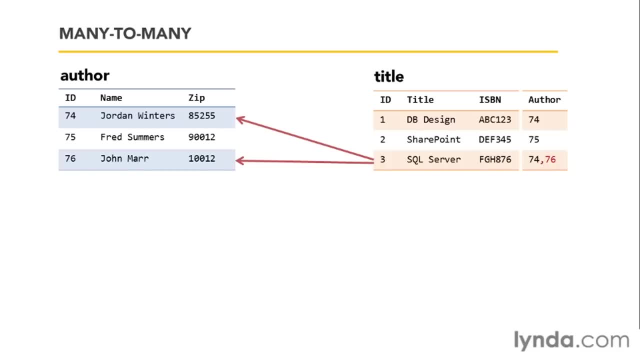 something quick and dirty And I'll just slide in a little set of comma-separated values there so that the author column can point to the title table. And I'll just slide in a little set of comma-separated values there so that the author column can point to both 74 and 76.. But that's just a cheat And 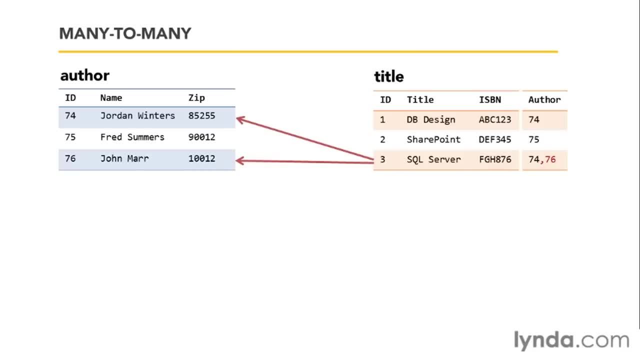 like adding a new column. this is not suggested either. In fact, we're going to solve this problem by getting rid of the author column entirely. So we go back to two completely detached tables, And what we do to fix this is we add another table. We add what's often referred. 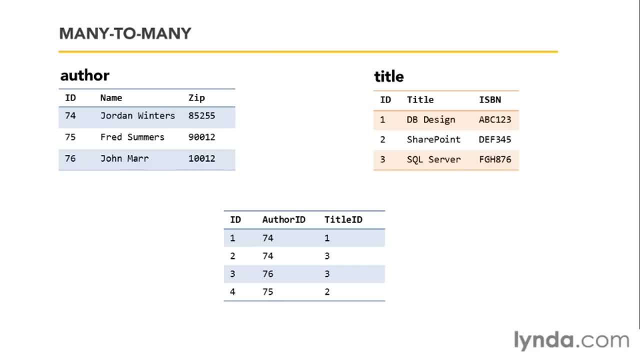 to as a junction or linking table. Now, the only reason for this table to exist is to join author and title. So we're going to add another table And we're going to add another table And we're going to add another title together. So, in fact, the name of this title by convention would be: 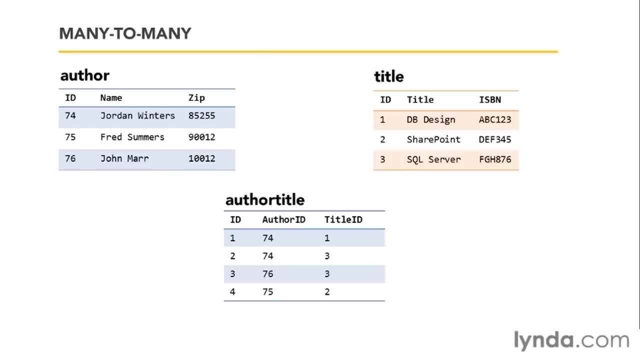 author-title Could also be title-author. It doesn't really matter which way around it goes, Because what we're going to do is set up two one-to-many relationships. In fact, you cannot, in SQL Server or in any other relational database you cannot- express a many-to-many relationship. 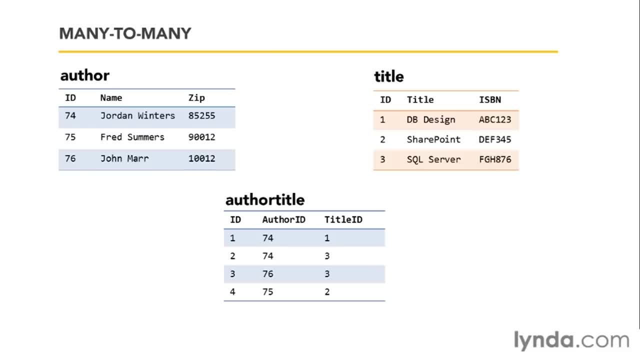 directly. You can only do two one-to-many relationships. So what we'll do is we'll define a one-to-many relationship from the author to the link table And we're going to do that by adding a title to author-title, So one author with ID 74 can exist in the author ID foreign. 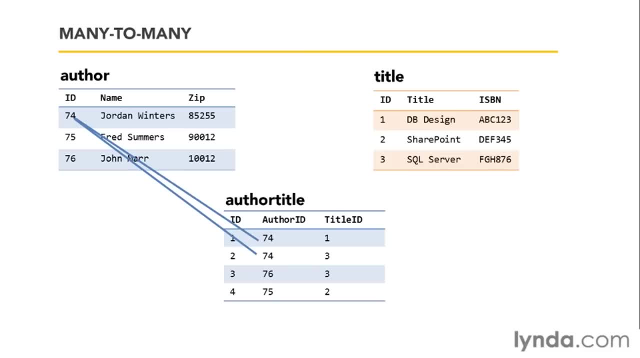 key column in author-title twice or three times or five times or a dozen. Using that, we can go from author to author-title, find a title ID and map it up to the title table, And we can also go the other way. We can take the identity of a title like number three, take it back to the 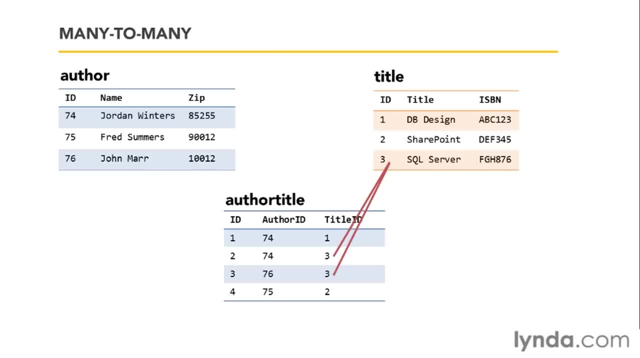 author-title table to two rows. there It's a one-to-many relationship. back the way, Grab the author ID and follow that back up to the author table. So we are expressing now a many-to-many relationship. And if you go looking in, say, some of the sample databases, whether 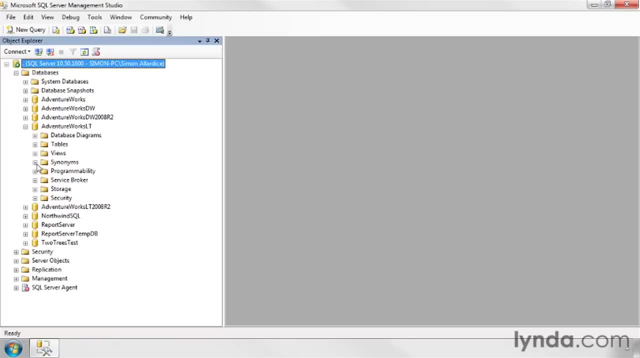 it's the larger ones, like AdventureWorks, or even the small ones, like AdventureWorks LT. any time you see a table name that seems to join the name of two other tables. so we have product model, product description and then product model product description you can make. 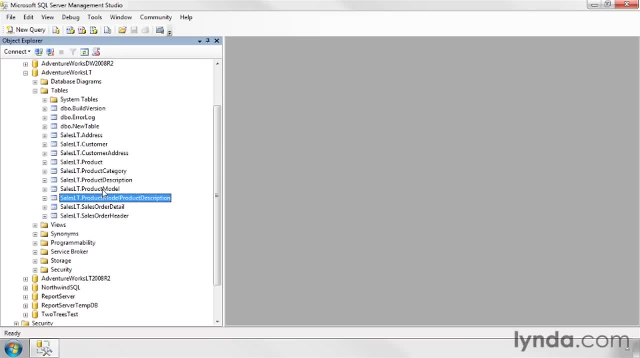 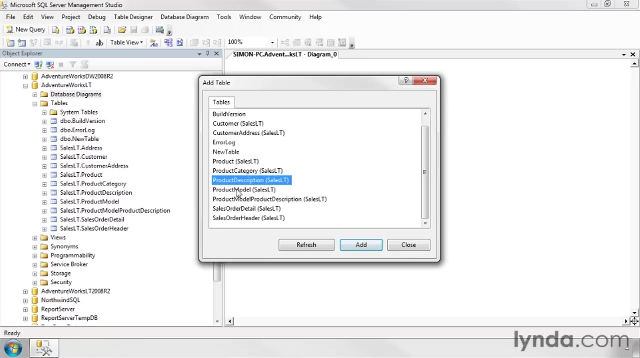 the assumption that the one with the longest name is the one with the longest name And if you want to confirm that, what we could do is make a new database diagram. I'm going to add just those three tables that I suspect that from product description I'll hold down control select. 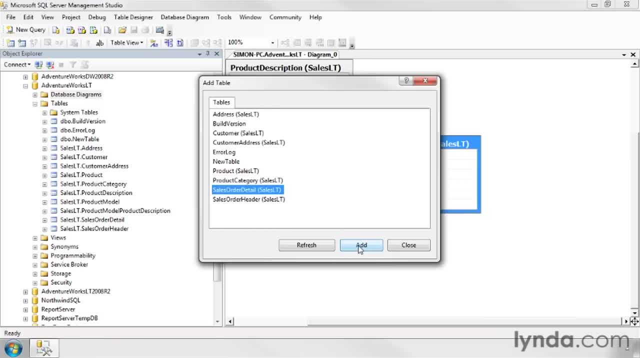 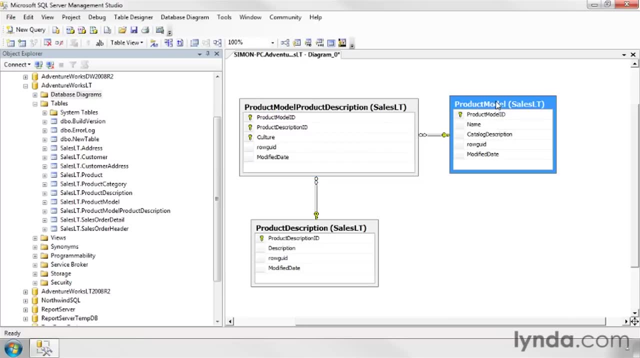 product model and product model product description. Click, add, Close this And what I can actually see here is my many-to-many being rendered out. We go from product model is the one to the many of product model. product description. Product description is the one to the many The. 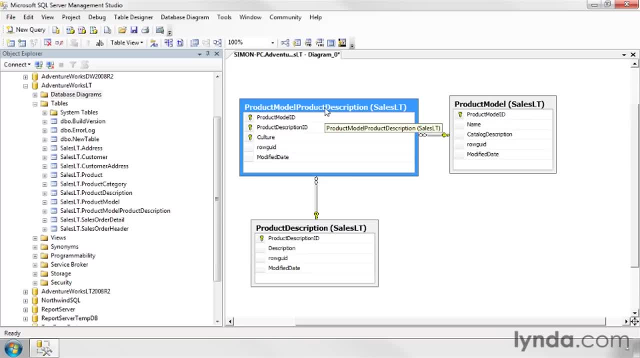 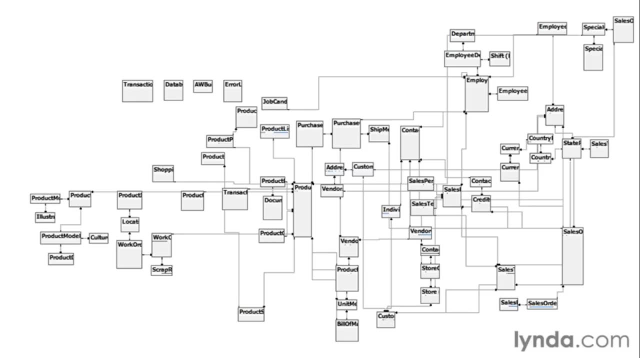 only reason for the existence of this table is to join the other two together In a large database. you're going to end up with a lot of one-to-many relationships between your tables, And a few of those will really be used to create a many-to-many relationship. Now, officially, there's also a 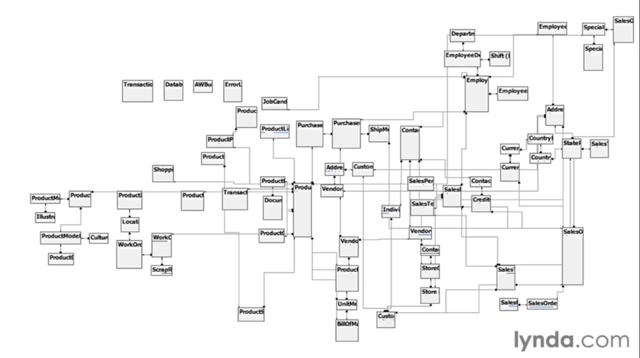 one-to-one relationship. that is possible, but it's not common at all. If you think about it. if one row in one table is pointing to one row and only one row in another table, well, you might as well just combine them, so it's. 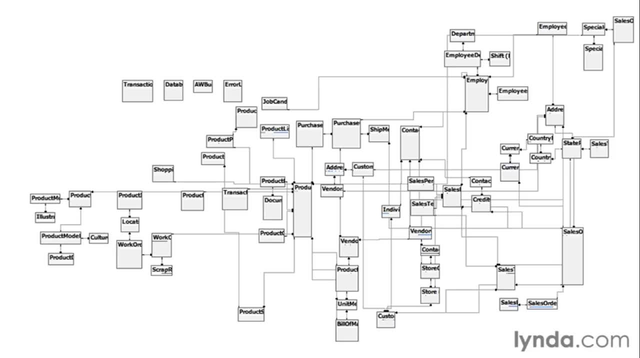 just one row in both places, Although also bear in mind that if those are the official three kinds of relationships- one-to-many very common, many-to-many quite common and one-to-one not common at all- you also have what some people consider a fourth kind of relationship. Zoom into 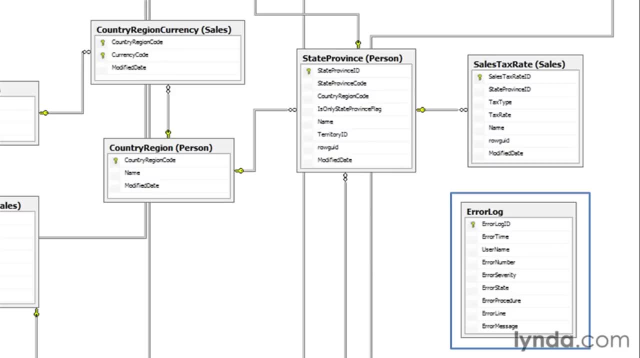 any large database diagram and you'll find things like this: a table just existing, without any. Some people consider none To be a relationship. If you get obsessive about what these relationships are- and again the geek trivia term is the cardinality is what we call something that describes the relationship between